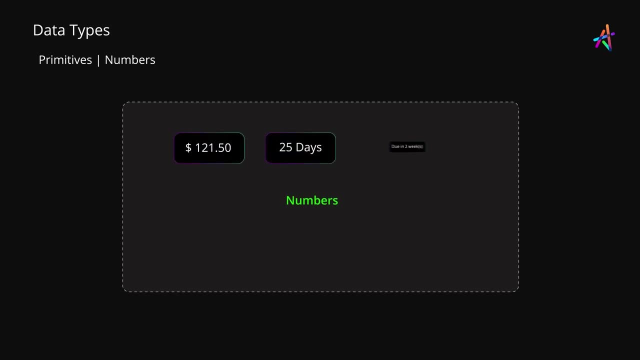 First up are numbers, So everything from cost of a product, number of days and weeks, temperature, number of emails in your inbox, the amount of money in your bank, your credit card number- all of these are examples of numbers. Numbers are often broken down into two or more. 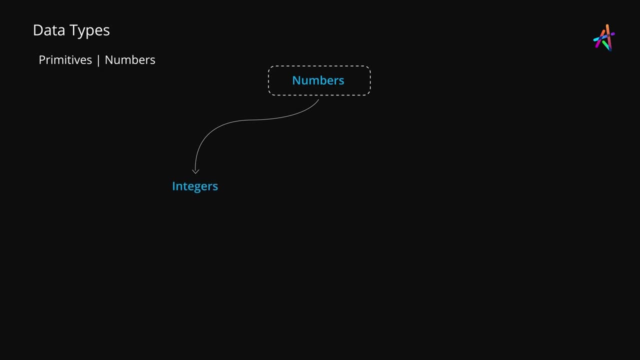 discrete types. For example, integers, are whole numbers that do not include a decimal point. These are great for expressing the components of a date, such as the day, month, year, your area, zip code, phone numbers, bank account numbers and so on. 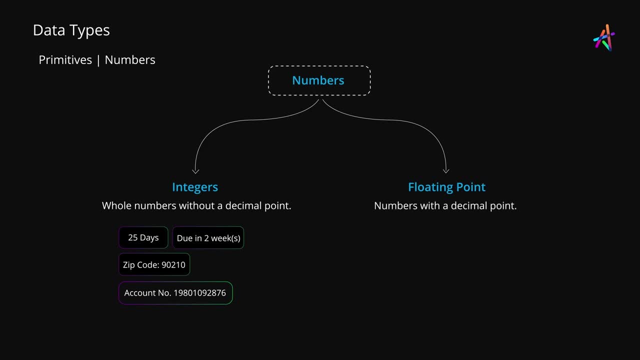 Likewise, floating-point numbers or floats are used to express numbers with decimal points, So the value of pi or time, temperature, etc. The lógical definition of the quantum number is basically the equation where the Width, cost of a product, dimensions of an object, distance between two points, amount of money. 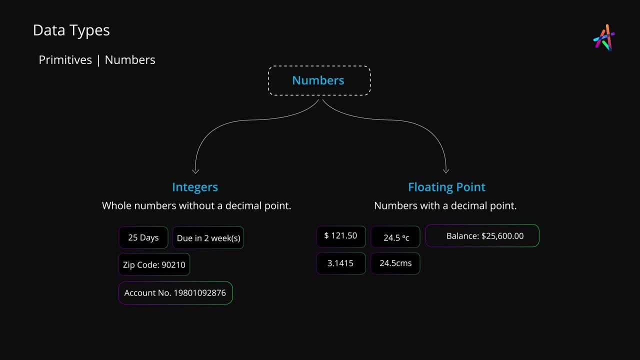 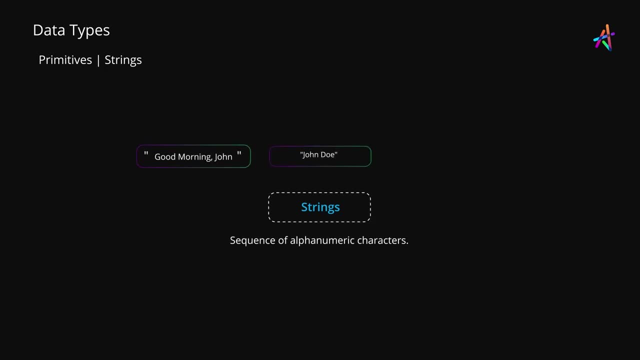 and financial data, and so on. Next up, we have strings, which are essentially a group of characters, and you can use strings to represent names, social media posts, emails, email ids, postal addresses, blog posts and virtually anything that contains alphanumeric data. These are usually expressed: 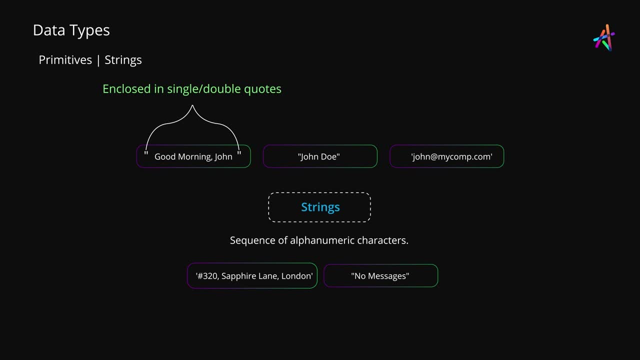 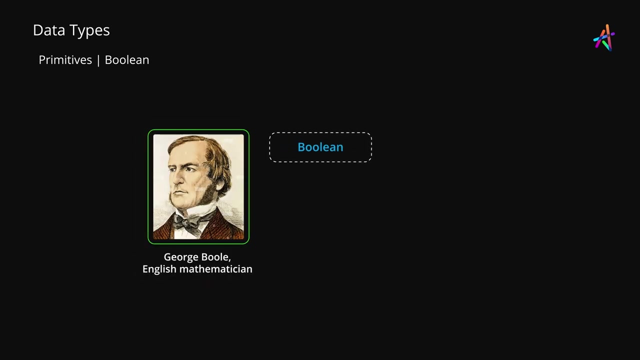 within a pair of single or double quotes. Some languages also include a type called char, which can be used for denoting a single character. Our next data type is called Boolean, named after George Boole, an English mathematician who, in his short lifespan of just 49 years, 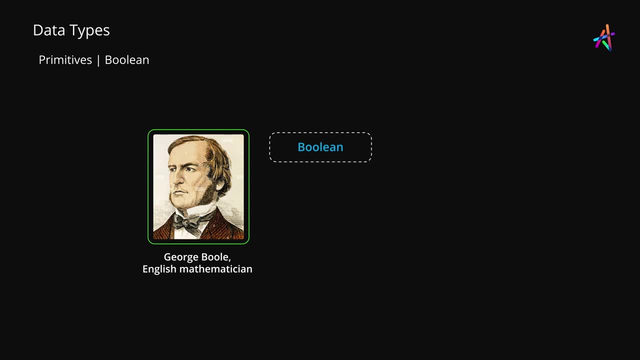 published several papers on mathematics, including the mathematical analysis of logic, which formed the basis of Boolean. Boolean values can either be true or false, and while this may not sound much, it is in fact quite useful when you need to express a switch, for instance, which should either enable or disable. 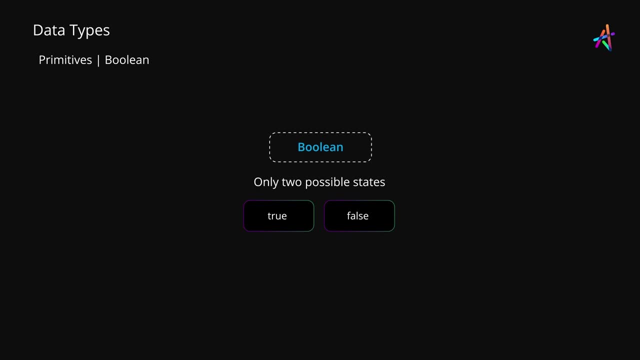 processing of some data. You also have decisions such as: is the temperature less than 15, or is this user registered or are you above 18 years of age? All these and similar questions can be expressed in a yes or no, or true or false.